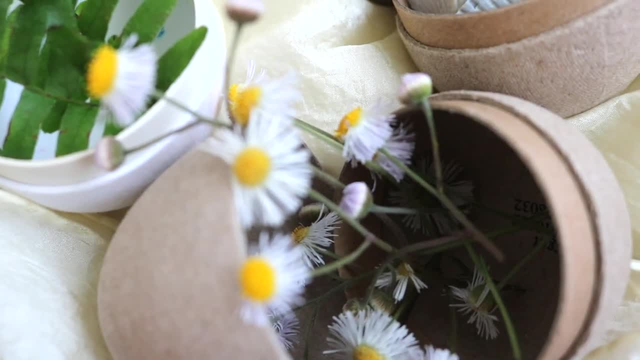 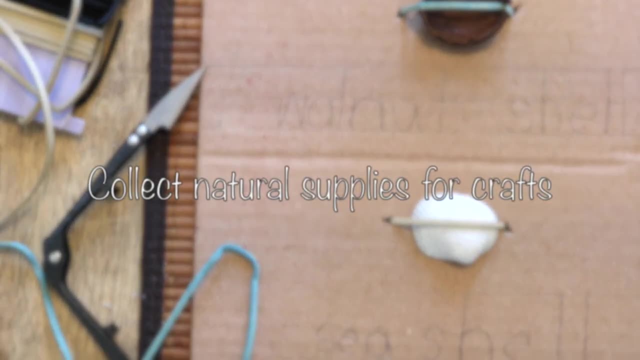 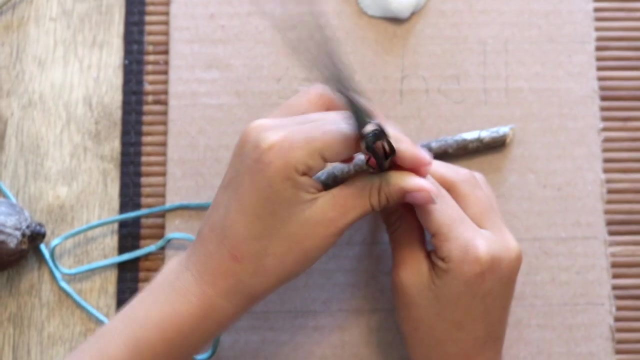 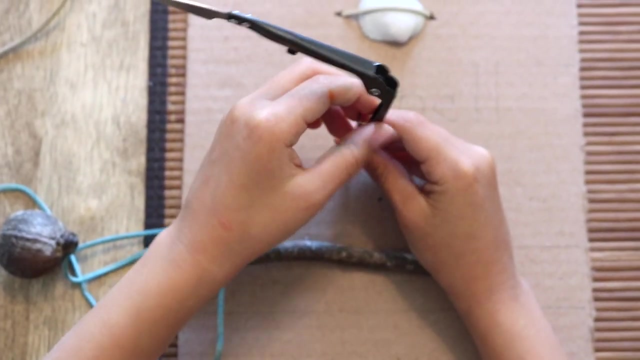 some beautiful nature treasures to display on this corner of magic. Just as much as we love collecting nature's treasures for our nature table display, we also love collecting treasures for crafts. There are so many crafts, so many ideas that you can find on Pinterest or several craft books that you can find online. inspired by nature. 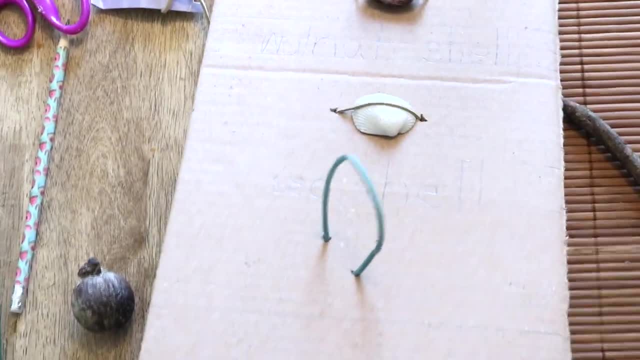 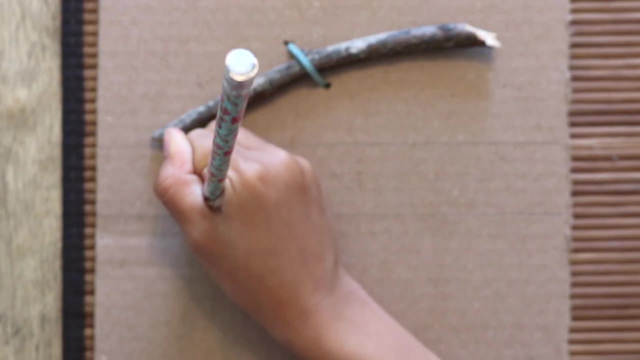 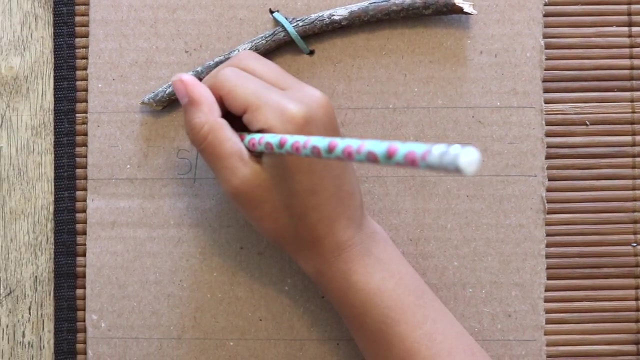 And before I forget to mention it, there will be a part two of this video where I share our favorite books and resources, not just for nature crafting, also for nature studying and just resources that inspire us to get outdoors in general. But one of our favorite crafts is a super simple craft that will motivate. 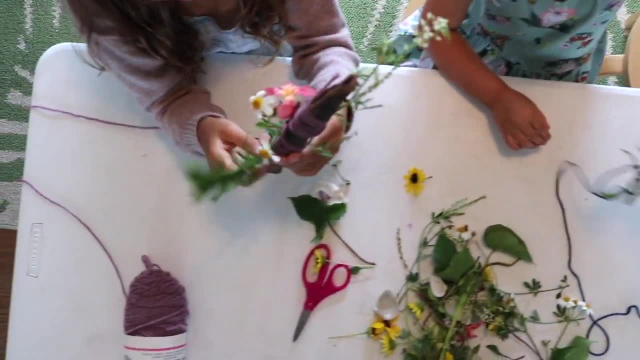 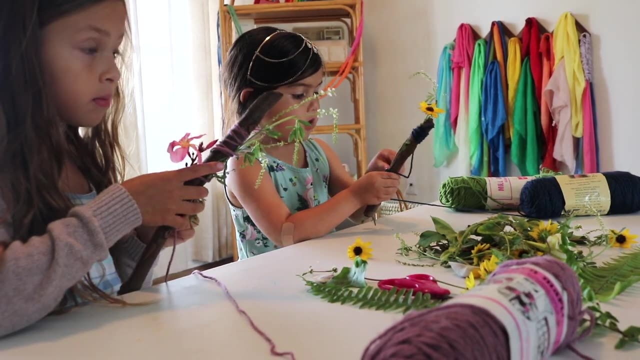 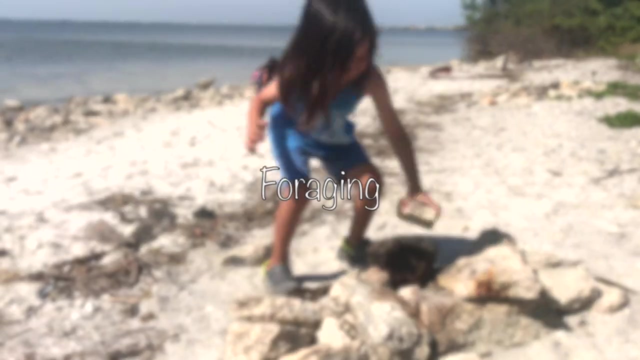 your babies to get outdoors. So collect treasures like wildflowers, twigs, interesting stones and leaves, seashells, And when you get back home, attach them to a stick with yarn and you've got yourself a treasure stick or wand. 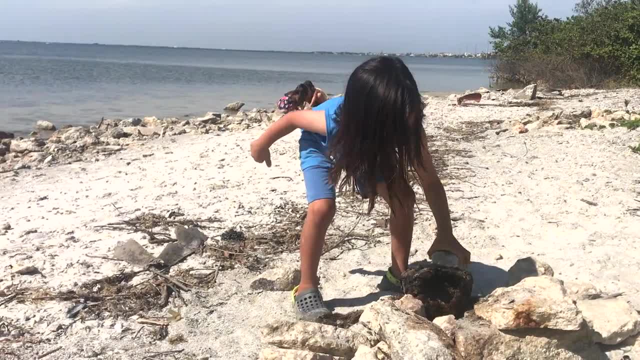 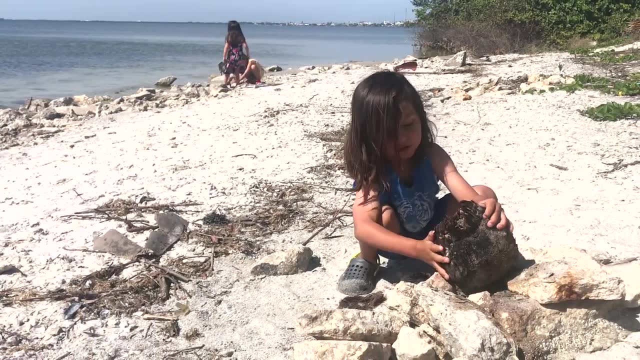 Our family picked up foraging about two years ago, and it's one of our favorite hobbies to do outdoors, So we're going to show you how to do it. I will say that before you begin to forage for plants, or fruits you'll be consuming- 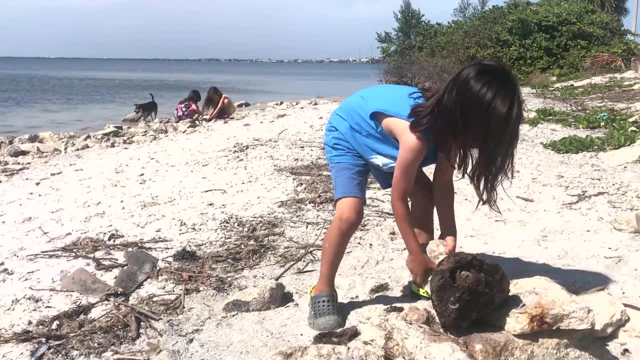 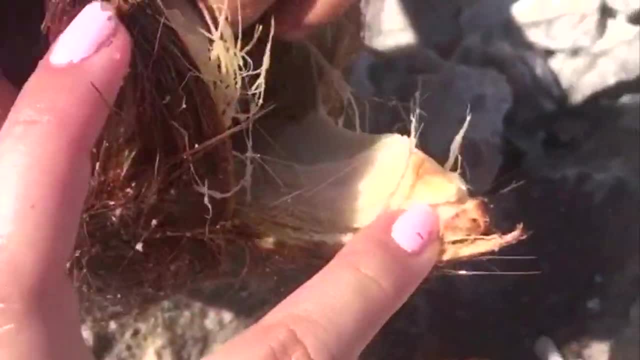 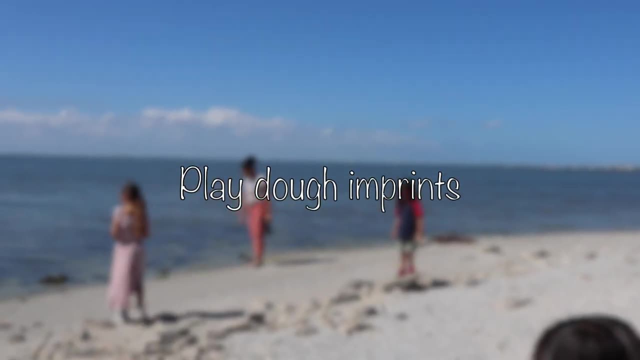 you should purchase yourself a guide or a book for foraging. in your specific region, We've foraged wild oranges and blueberries, blackberries for juices, edible flowers for salads and wild coconuts. I'm pretty sure that my youngest would vote. 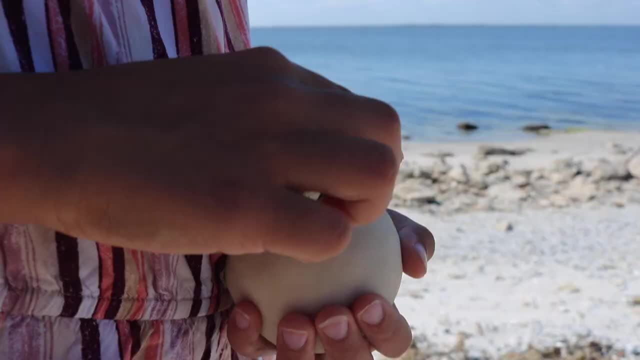 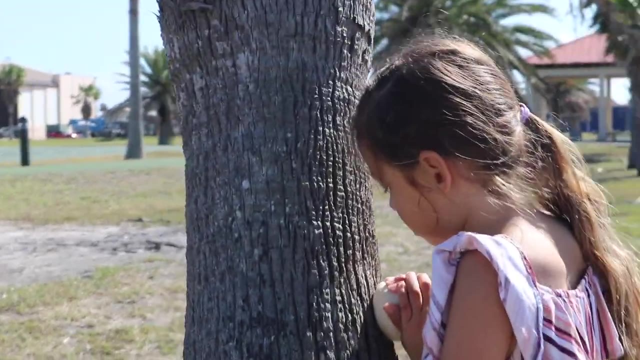 on Play-Doh imprinting as their all-time favorite nature walk activities. We provide everyone with a ball of our homemade play-doh and, by the way, i am going to leave a recipe to our dough down below. it's the best recipe we've tried and i guarantee you'll never purchase play-doh. 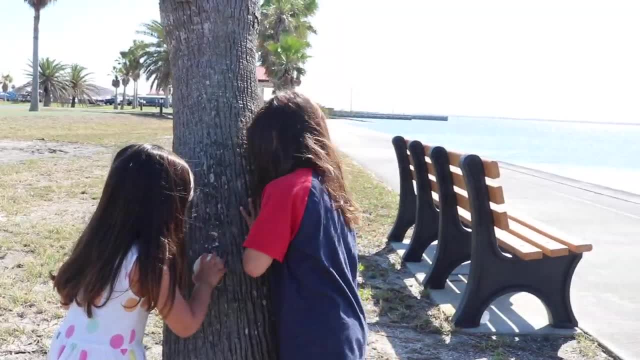 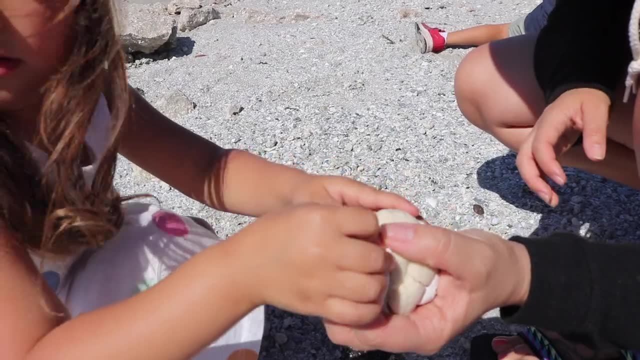 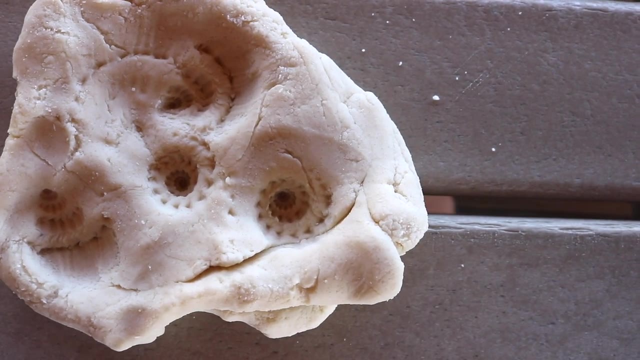 again, as i was saying, each person will carry their ball of dough and we'll bring it on a walk with us and just find interesting items in nature to imprint in the play-doh. guarantee your littles will get super creative with this, and it leads to discussions of patterns and textures and symmetry. 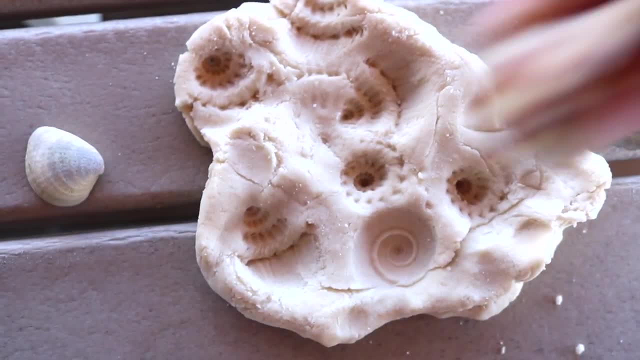 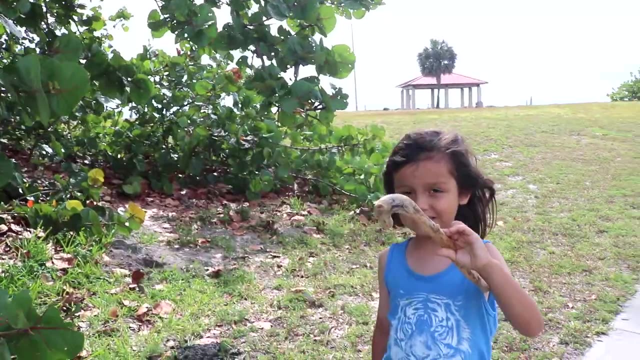 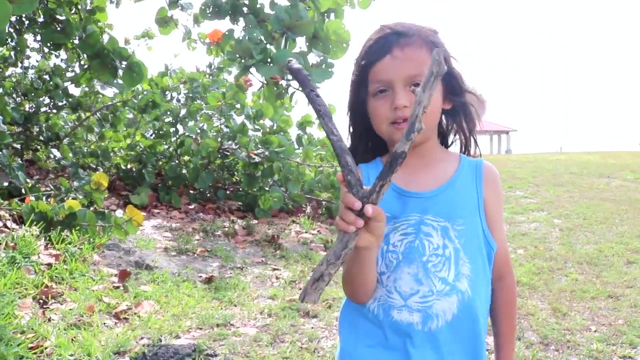 just such a fun activity. our family has this little game where we're always looking for letters in nature. you'd be surprised with the interesting findings you'll come across. we keep a list of the letters we have found so far, and while it may be a while before we find the entire alphabet, 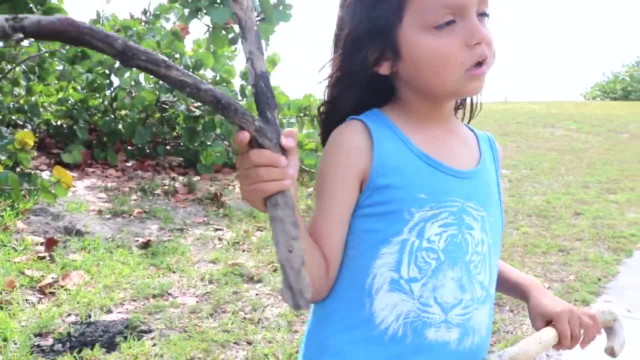 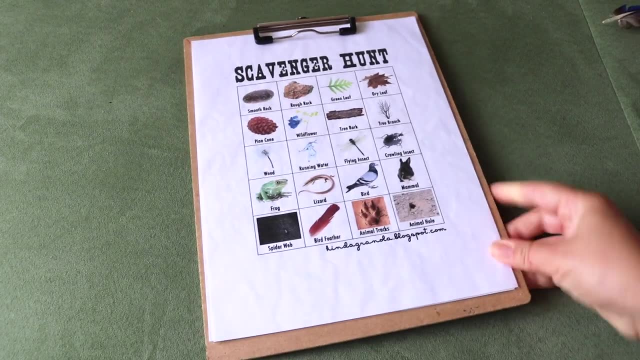 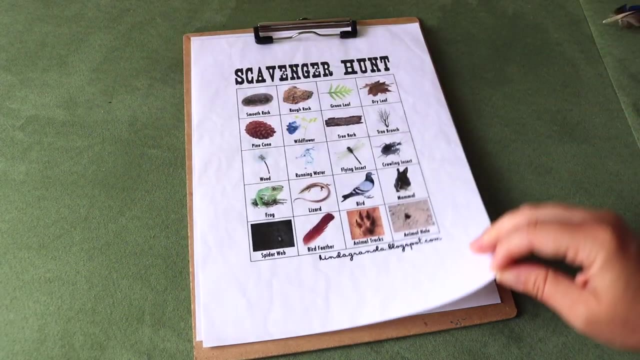 it's a fun nature game we have going on like like jacob jacob, jelly jam, scavenger hunt. scavenger hunts are always a big hit and open-ended. there are so many variations and possibilities. you can find free printables online, along with inspiration for super neat scavenger hunts. you. 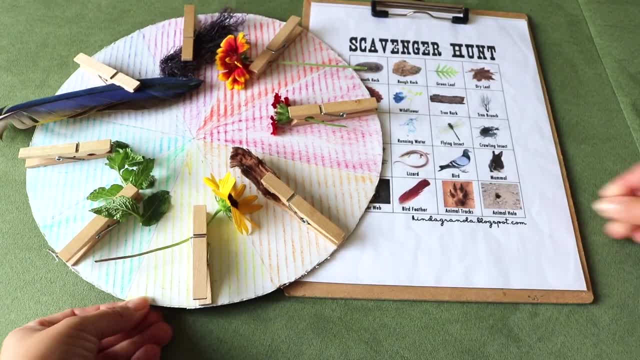 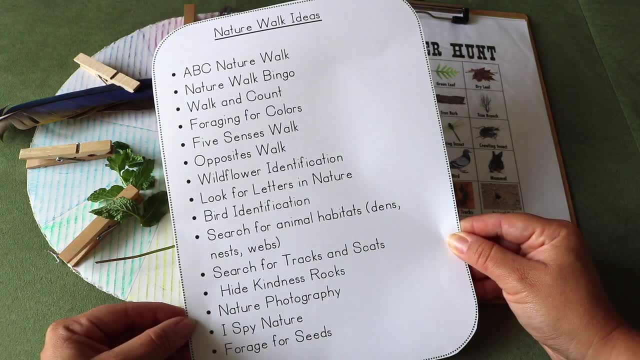 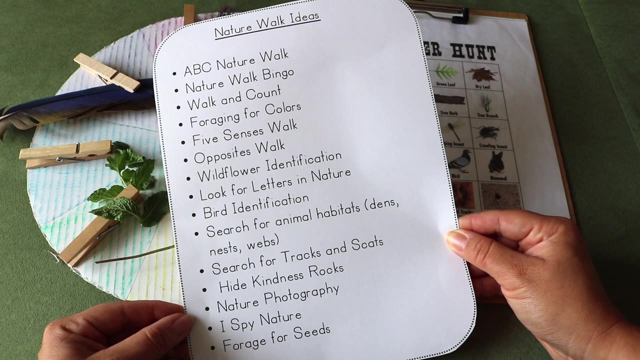 can create on your own. many don't even require from much planning or bringing anything along, like an abc nature walk. how many things can you find in nature that begin with the letter a or b or c and so forth? uh, nature walk, bingo, walk and count. foraging for colors a. 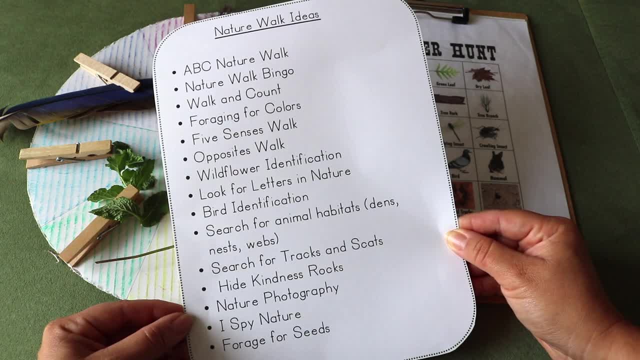 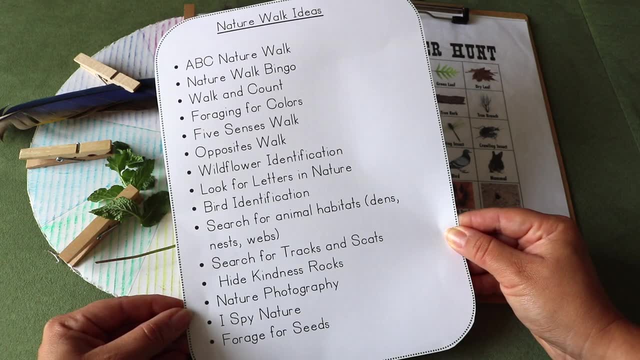 walk and a walk and turn at least one of the five senses. walk- what do you see, what do you hear, what can you taste and touch? searching for animal habitats like dens and nests is one of our absolute favorite activities. when we don't want to bring anything along an opposites, walk is. 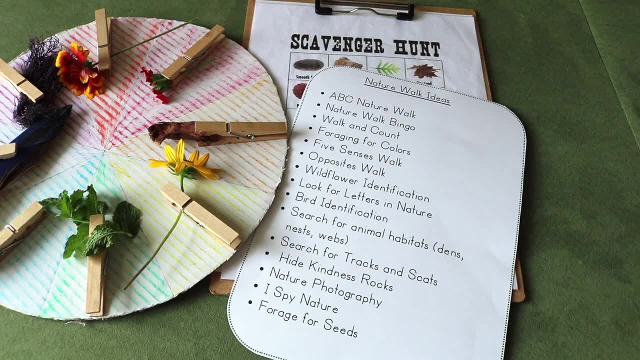 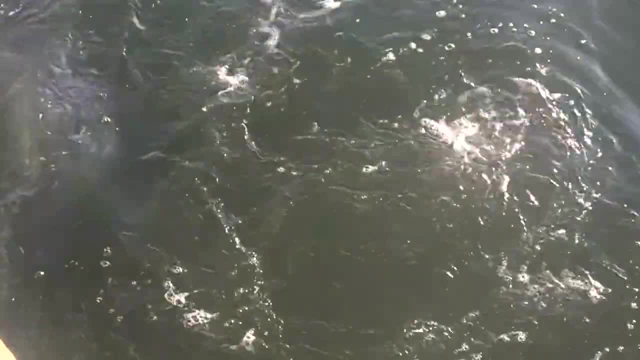 always fun. find something that's rough, find something that's smooth. i strongly and passionately believe that teaching our children about the natural world should be treated as one of the most important events in their lives if we want our kids to be successful. we can make a better day or night. and we should have a good time during these three whole years. so let's continue this scientific vibe and give a makeover of the places we can't miss and make sure that we definitely get the right notes for so many more year to come as we continue to get into this game science adventure. I hope you'll enjoy watching and I'll see you next time.